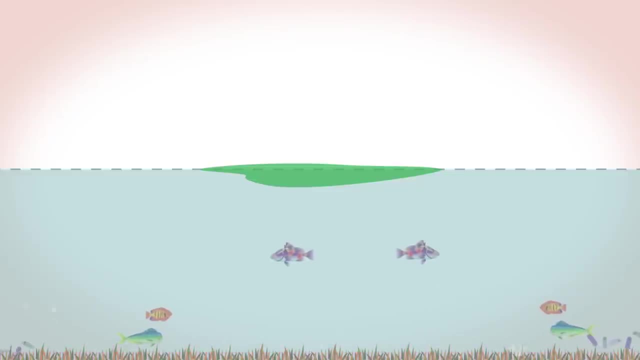 from the vegetation deeper down, which dies. Bacteria then feed off the dying vegetation and use up the remaining oxygen supply. Once the oxygen has gone, all animal life dies. The lake ecosystem is destroyed If heavy metals such as lead, mercury and cadmium get into rivers. 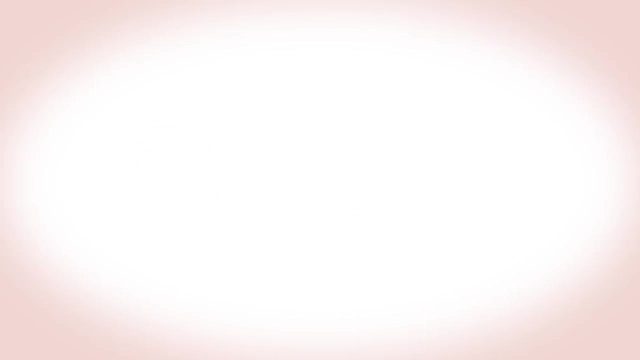 and lakes, many animals will die. In Minamata, Japan, a polluting mercury fungicide factory was closed in 1968, yet people there have continued to be affected by the mercury poisoning, the so-called Minamata disease, ever since. 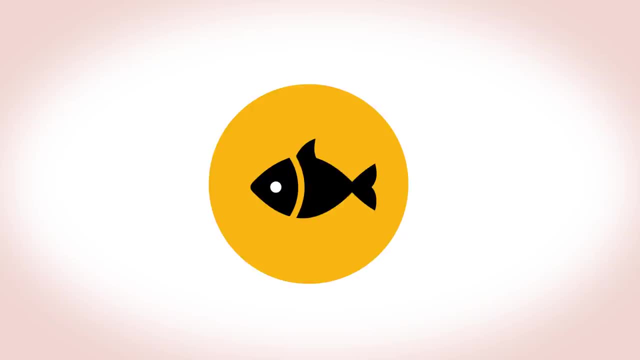 because the fish caught locally in the bay still have traces of mercury in them. Nowadays, the use of mercury and cadmium in fungicides has been largely replaced by copper and organic compounds. The removal of lead from petrol, which is also used as a source of mercury, has also been a key factor in the 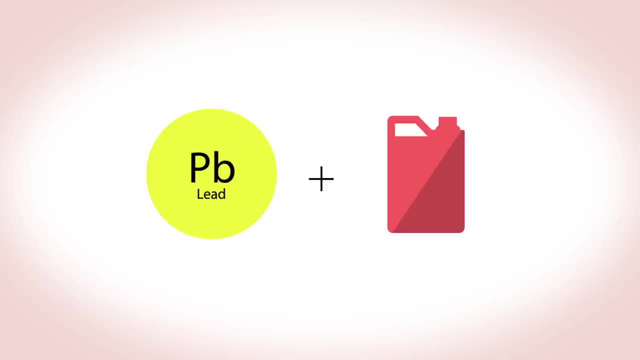 resulting lead poisoning. Since then, the use of lead has become more widespread. Theohl began in the 70s, when it became clear that lead poisoning, causing mental defects, was caused by the lead compounds added to petri l to make it burn more smoothly. It has taken 40 years since then for a United Nations global ban on the sale of leaded petrol. The last six nations complied in 2013.. Radioactive waste is normally stored above ground in water tanks, waiting for a single drop in the amount of oil they need, and the amount of oil used is nearly half the amount that is needed to produce oil. Radioactive waste is normally stored above ground in water tanks, which is only used when a plant, as well as many other kinds of cells, are working. 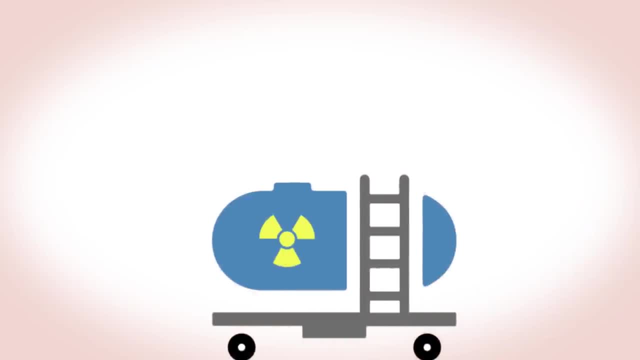 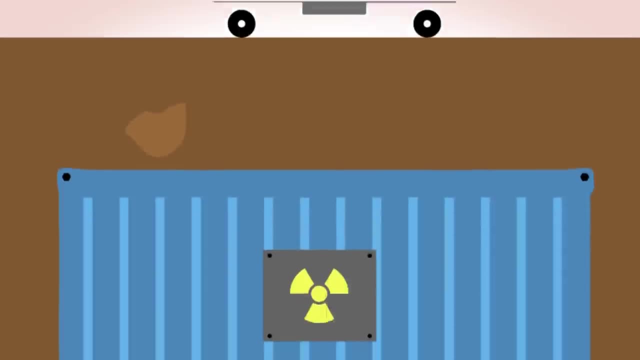 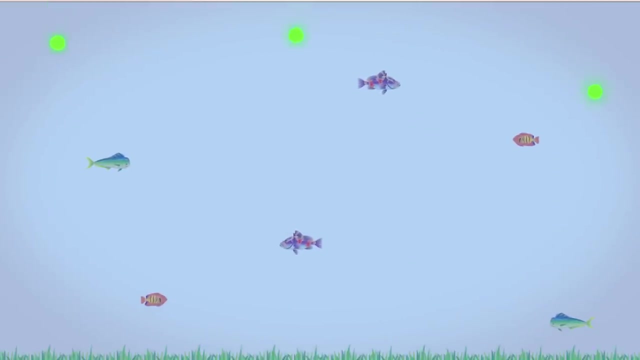 is normally stored above ground in water tanks, waiting for more permanent underground storage, where it has to be safe for millions of years. There are fears that these underground stores could fail and contaminate watercourses. Currently, small amounts of radioactive material are allowed to be washed out to sea. 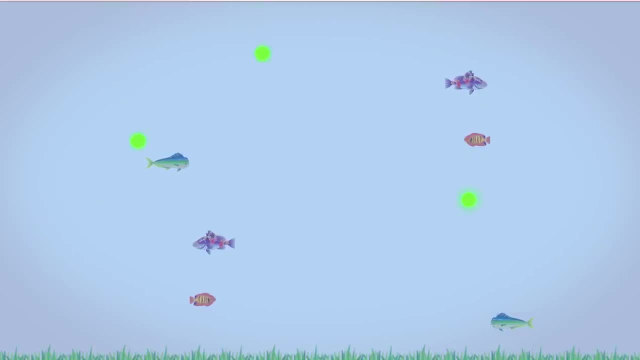 on the basis that it will become so diluted that it will make no difference to the natural background. radioactivity in the oceans Following a nuclear disaster like Five Mile Island in 1979, Chernobyl in 1986 or Fukushima in 2011,. 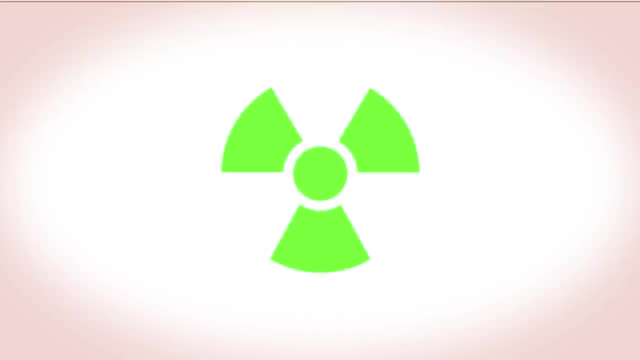 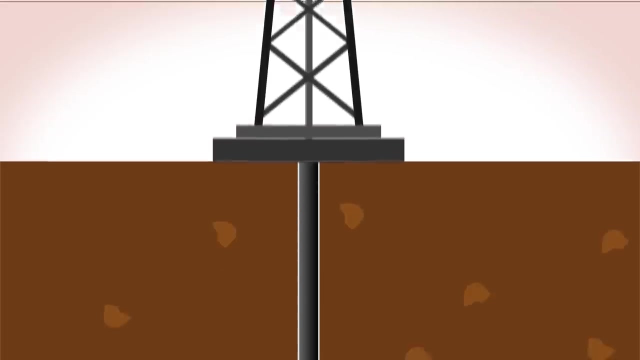 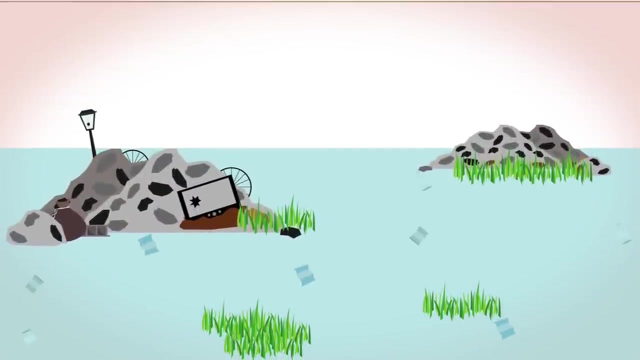 watercourses and the oceans can become dangerously polluted with radioactive waste During mining and drilling operations to extract minerals from the earth. aquifers, which are the underground watercourses, can become polluted. Huge amounts of plastic are thrown away from ships and washed out to sea from rubbish dumps on land.